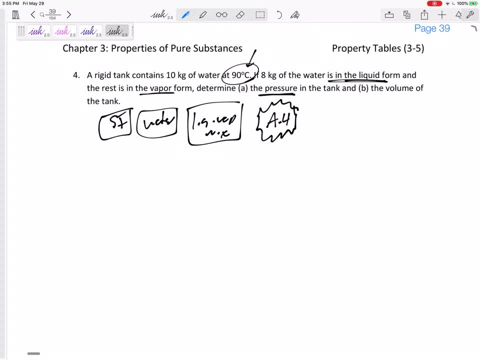 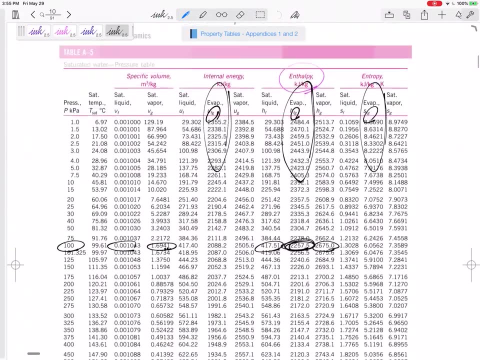 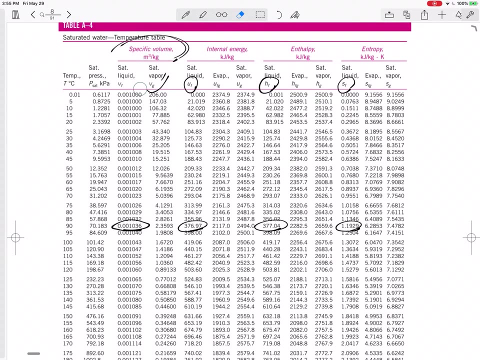 It's a one-to-one right, And so I would go to this temperature and I would find P sat for 90 degrees C. I think we actually did this table All right, so 4. Water. so I'm in Appendix 1.. 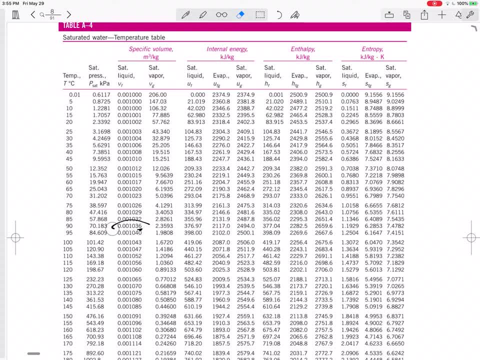 I'm in water, so I'm in 4,, 5,, 6, or 7.. It's saturated, so I'm in 4 or 5. And I'm given the temperature, so I'm in table 4.. 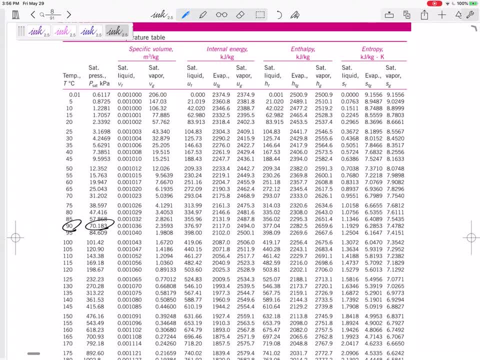 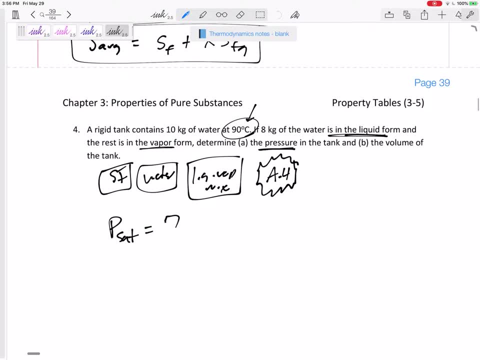 90 degrees C. that is the saturation pressure. That is the pressure: 70.183.. 70.183.. Go back and look at the units. They were kPa, kilopascals. Okay, then the volume of the tank. 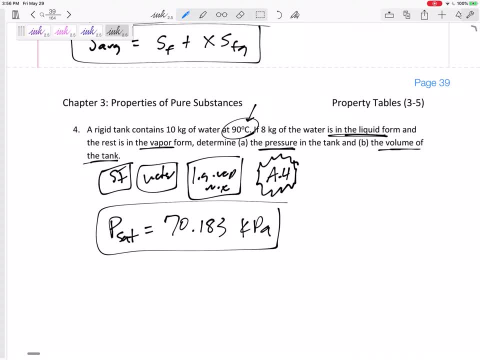 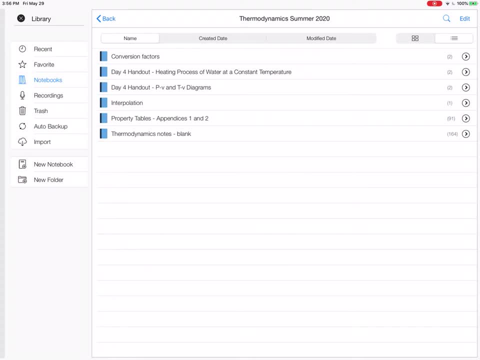 Then the volume of the tank. Well, the property table's not going to give me the volume of the tank, but I bet you, the property table could give me the specific volume of the tank. right, The property table's not going to give me the volume, but it could give me the specific volume. 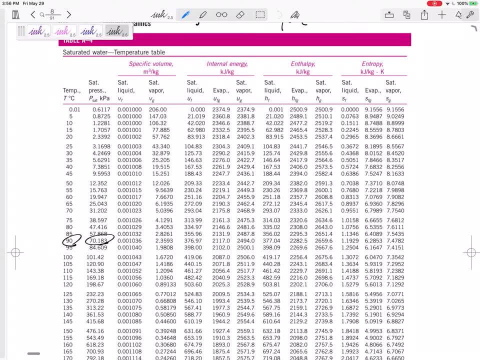 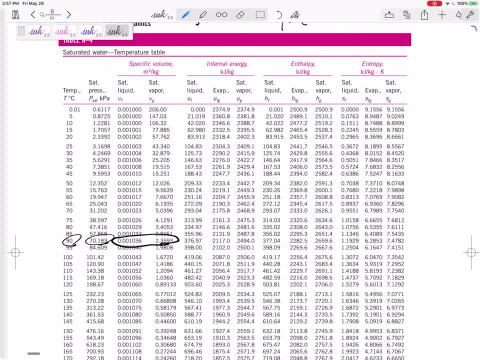 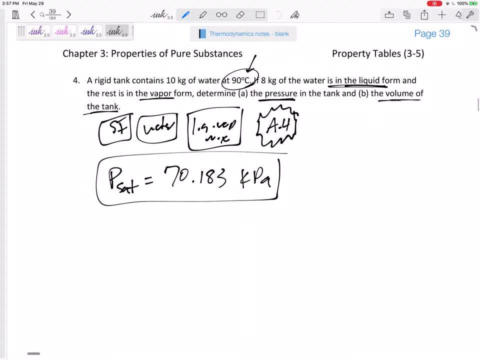 Yeah, it's somewhere in between the two. How far in between the two. I need to calculate the quality X. I need to calculate the quality X. So the quality X is mass vapor over mass total, Not mass liquid over mass total. 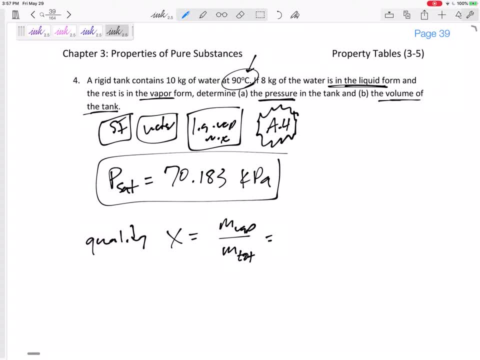 Not anything, Not anything else, but mass vapor over mass total. Write that on your formula sheet and double check. Make sure you're doing that correctly. All right, so this would be- let's see, All right, a total of 10 kilograms. 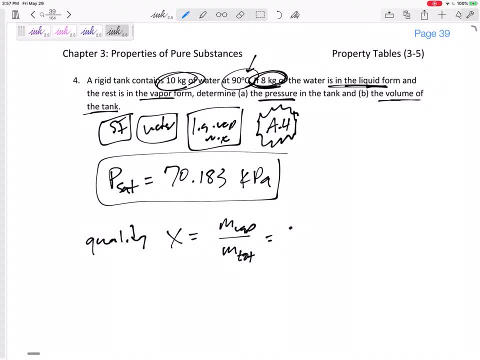 Eight kilograms is in the liquid form. So what is this? Two kilograms is vapor. Didn't explicitly tell us that, but we could figure that out Over. the total of the quality is 0.2, right If we have 10.. 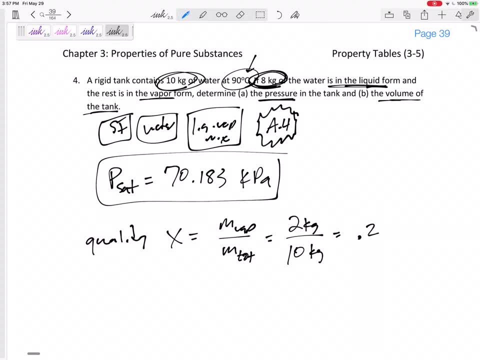 And eight of it is still in water. It only has a quality of 0.2.. It's 20% of the way in mass of going from liquid to vapor. So quality is 0.2, right X is 0.2.. 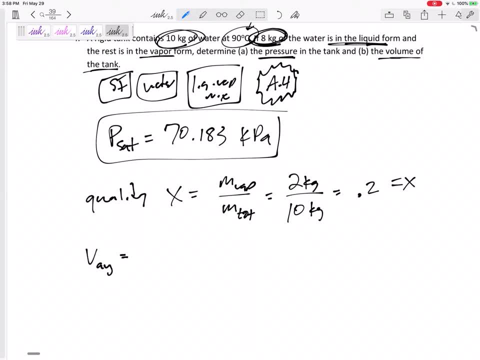 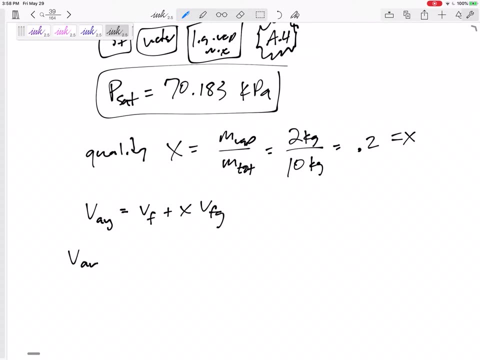 Now I bet I can get the average specific volume. That's not exactly what it's asked for, the total volume, but first I'm going to get specific volume. Average. specific volume is VF plus X, VFG, VF. all right, so the average would be VF. 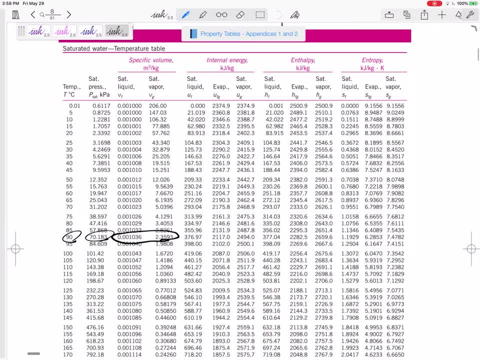 I go back to the property tables. VF is 0.001036.. VFG: this one doesn't tell it to us. just because these are so large and these are so small, This middle column would practically still be the saturated vapor values. 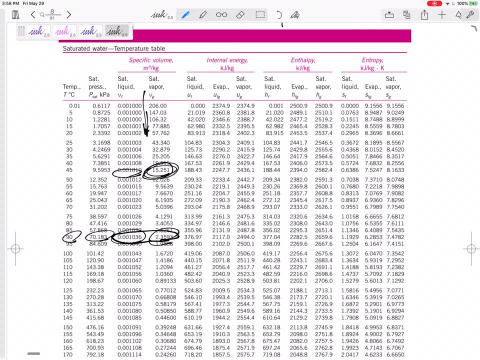 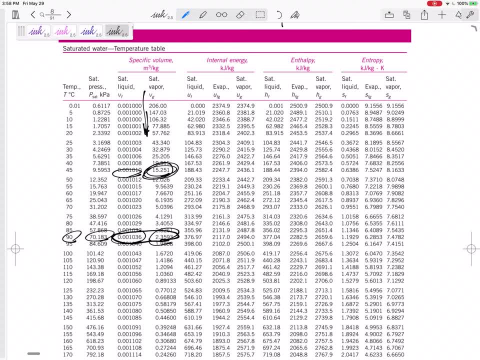 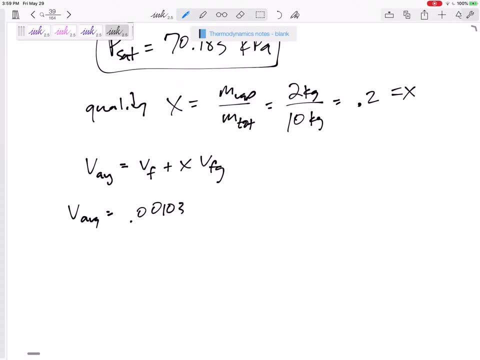 Okay, VFG. it's not going to really change your answer, but I like to subtract the two, So I'm going to all right. so there's VF, there's VG. so let me go back to our notes. VF was 0.001036, and be careful not to accidentally leave out a zero or something. 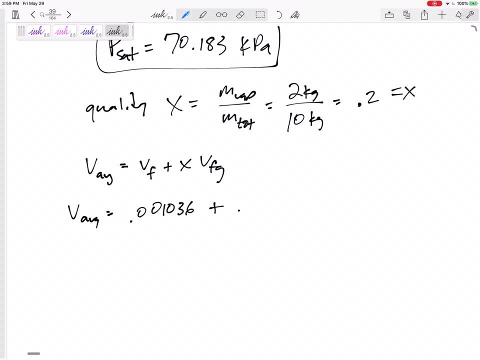 That would throw off your numbers a bit. Okay, minus quality times: VFG: All right, so we didn't have a column for VFG, so I want us to do this manual: 2.3593 minus 0.001036.. Yes, it's going to be practically 2.358.. Do that, Some would also. 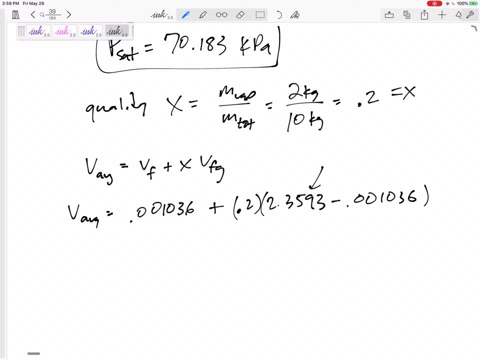 not care if you added this or not. I like us to do the same thing for every problem. V would be 0.473 meters cubed per kilogram. I was about to box that in. That's not exactly what it asked for. 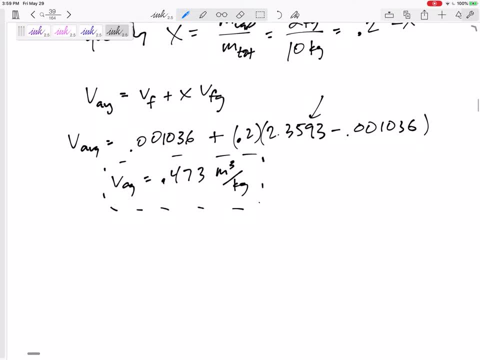 It didn't ask for the specific volume, It asked for the volume. So big V, let's see. V equals V divided by M. multiply it times the mass. Let's make sure those units make sense. If I take that, multiply it times the mass, I would get big V. yeah, 0.473 meters cubed per kilogram times the. 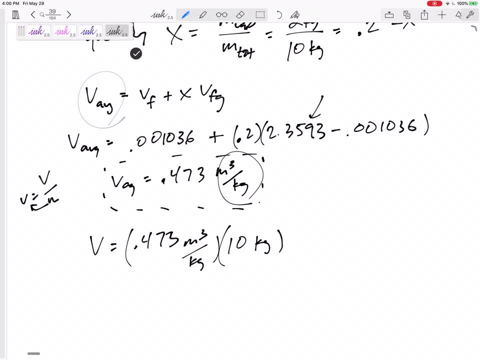 total, All right. so this is going to be 0.473 meters cubed per kilogram. So we're going to multiply it times the mass. So we're going to multiply it times the total, All right. so this is the average. If it were a homogeneous total, a full 10 kilograms and all 10 kilograms had that. 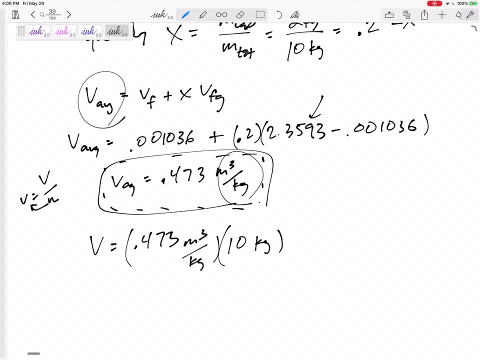 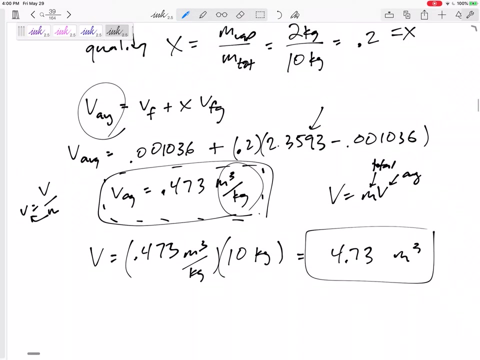 average specific volume. All right. so this, when I do V equals MV. this is the total and this is the average, right here, All right. 4.73 meters cubed. 4.73 meters cubed And you could have done this a little bit longer route. See if you get the same. 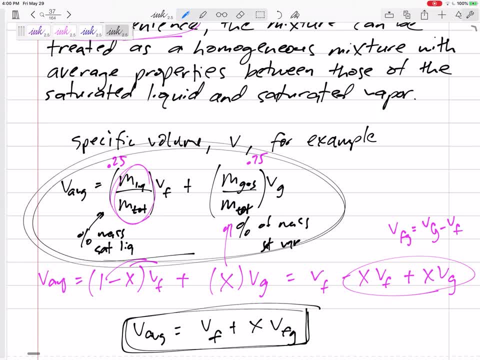 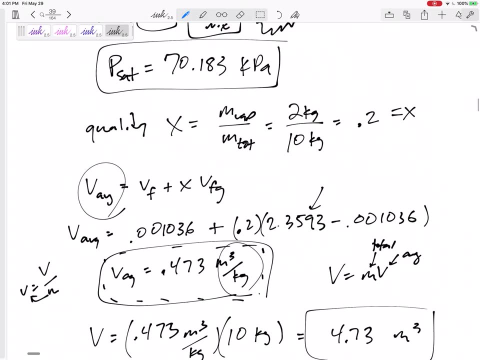 answer A little bit longer route. if you took that, you know, and if you said 0.8 times the VF value, 0.2 times the VG value and add them up, you'd still get 0.473.. All right, so let's take a. 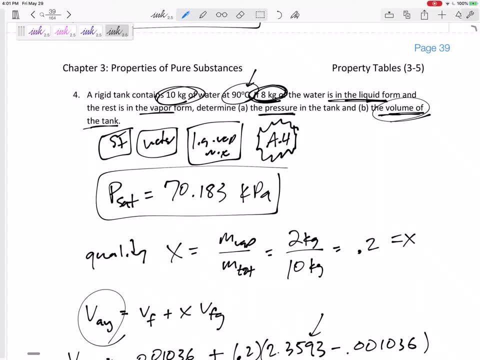 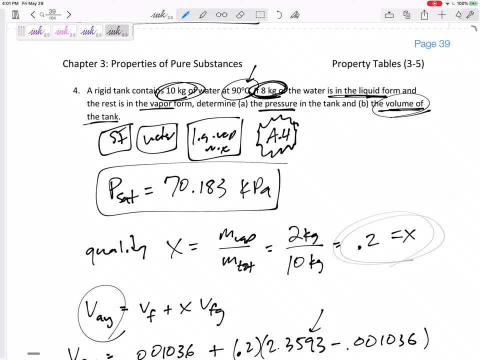 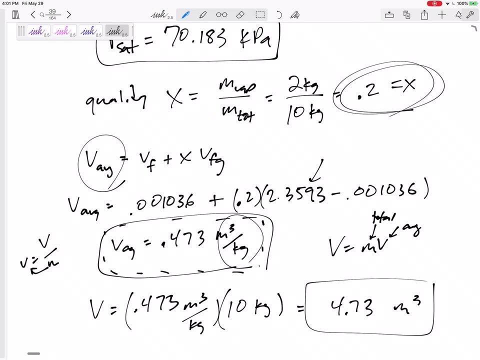 step back and look back. I had to make sure I was in the right property table. I knew it was a property table. I had to calculate the quality just by giving the masses that they told me. Then I used V equals VF plus X- VFG to find the average specific volume If it was a homogeneous mixture. 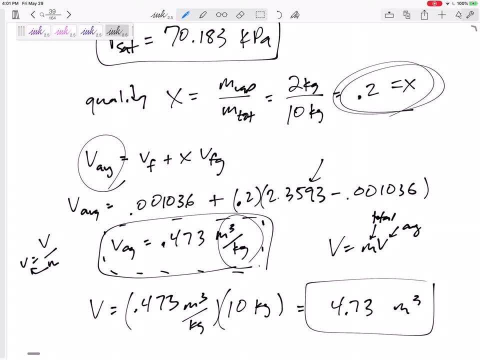 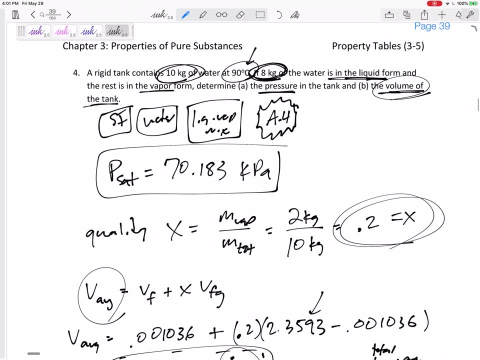 that all the particles had an average specific volume. of that, then I'd take the mass of all the particles to get the volume. Remember that you know property tables give you specific volume. Many times, though, you are asked for um total volume.